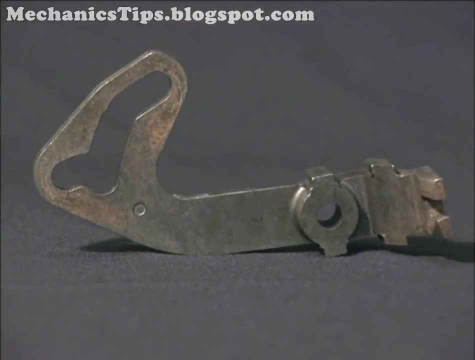 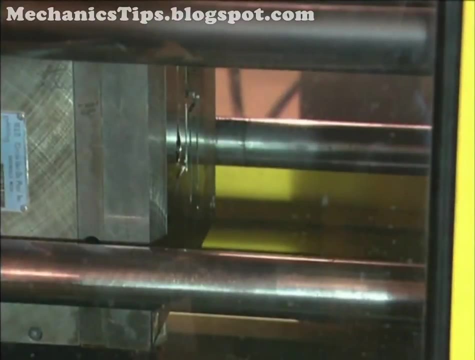 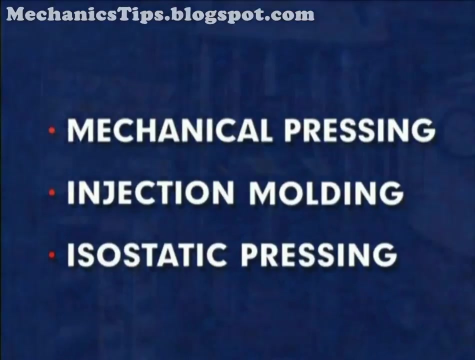 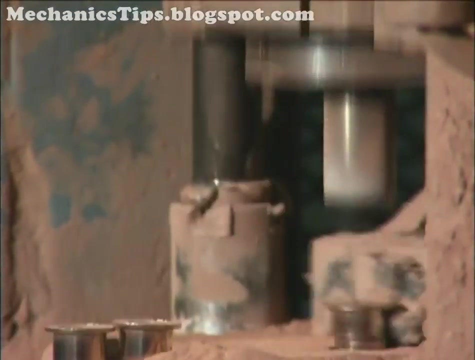 of structural parts increases directly with increasing density. The common methods of consolidating and shaping metal powder for parts production include mechanical pressing, injection, molding and isostatic pressing. Most parts are made by mechanical pressing and sintering. Parts are usually small to moderate in size and can be simple or complex in shape. They 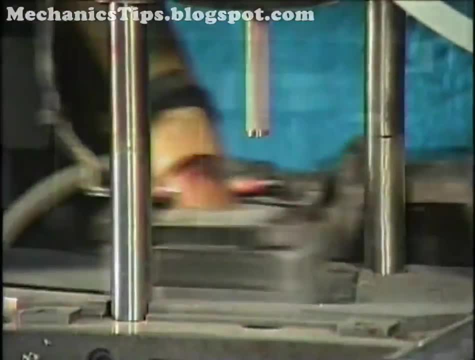 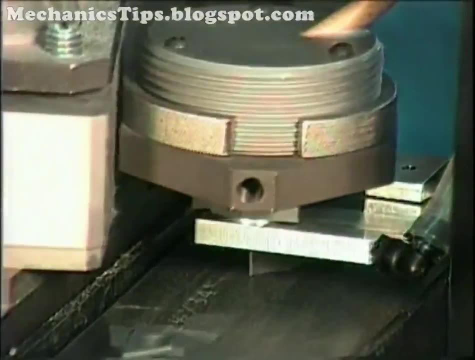 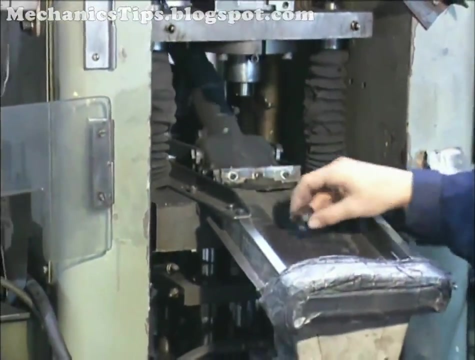 can be very thin or thick and can also have one or more levels, shallow or deep holes and various other details. Parts produced by mechanical pressing can be net or near net in shape and have very close tolerances. Part production rates are high from several 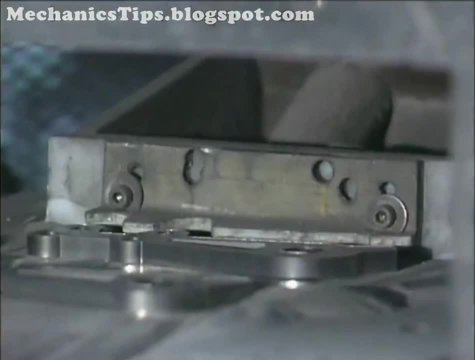 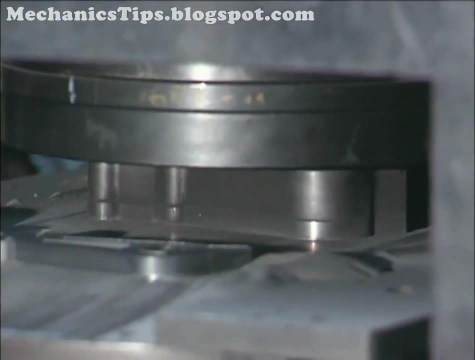 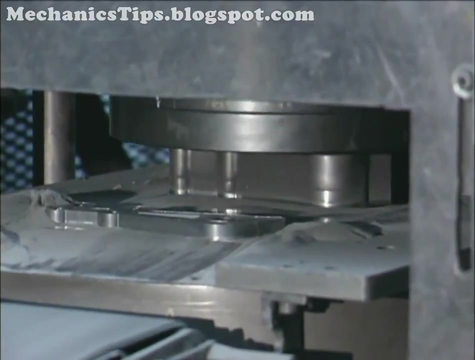 hundred to thousands of parts per hour. In mechanical pressing, the powder is automatically gravity fed into the die of a mechanical or hydraulic press and consolidated to a specific density. Pressures of 10 to 60 tons per square inch are created by the vertical action of an upper punch or by the double action of 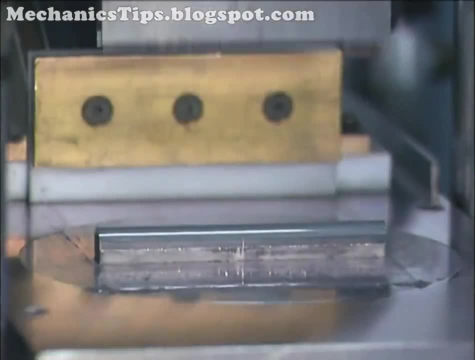 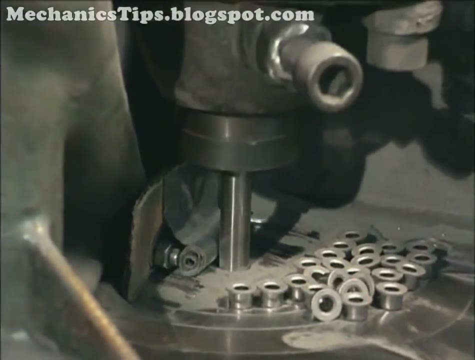 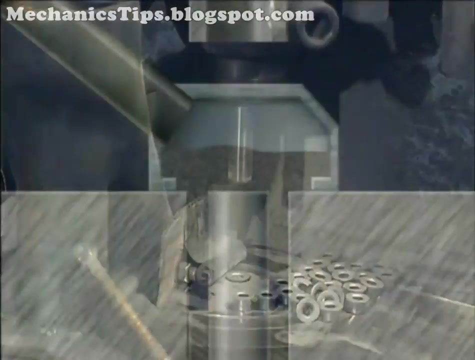 an upper and lower punch. Pressing is typically at room temperature, although the pressure is usually at the lowest level, Although elevated temperatures can also be used. Core rods are used inside the die to control formation of holes parallel to the direction of pressing. 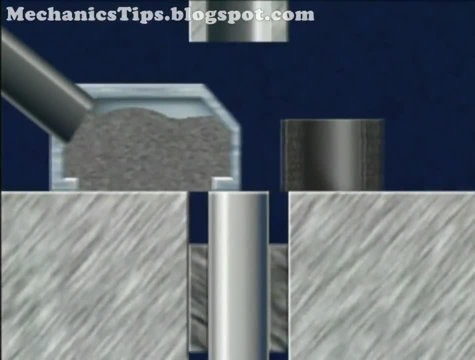 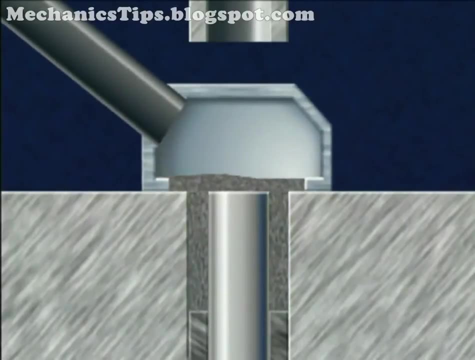 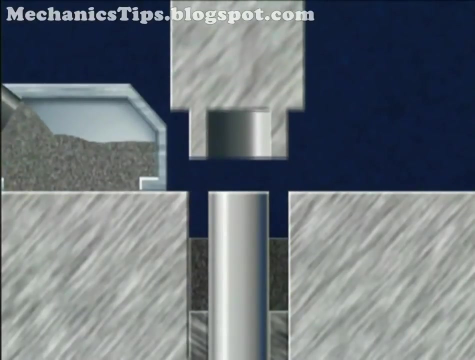 If the part being made is thin and uniform in height, the powder can be pressed from one side by the upper punch. When that punch withdraws, a lower punch raises the part out of the die. The part is then ejected by the wiping action of the powder feed chute, which 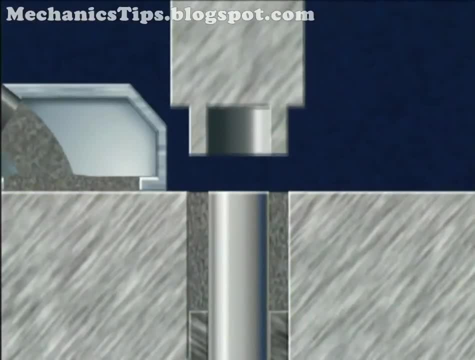 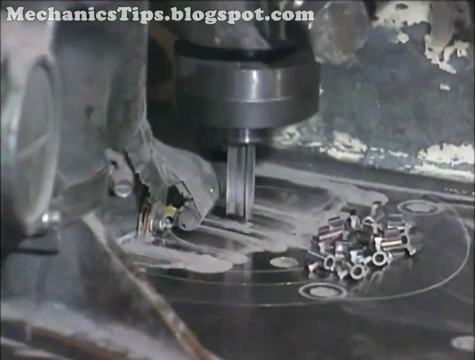 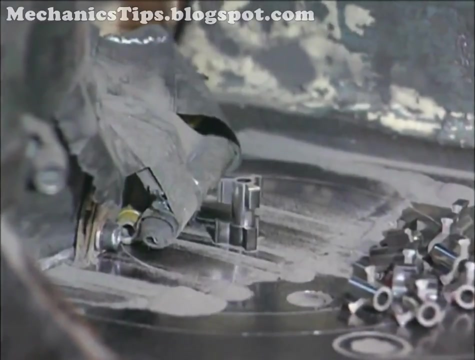 also wipes powder for the next piece into the die. Ejection from the press can also be accomplished using automated handling equipment. The density of pressed powder tends to decrease along part height as the distance between the compacting punch and die increases To produce more uniform density. thick parts: 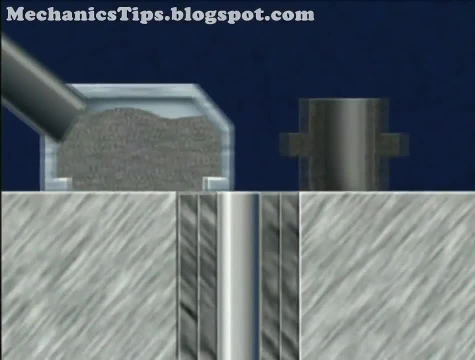 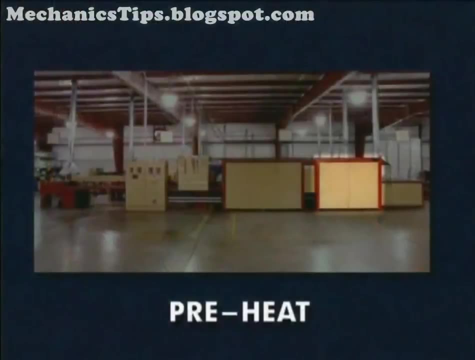 are compacted by a set of upper and lower punches. After pressing, parts are transferred to the center board furnace. sintering furnaces include preheat, high heat sintering and cool-down zones, each having a controlled atmosphere depending on the base metal of the part. the atmosphere of the sintering. 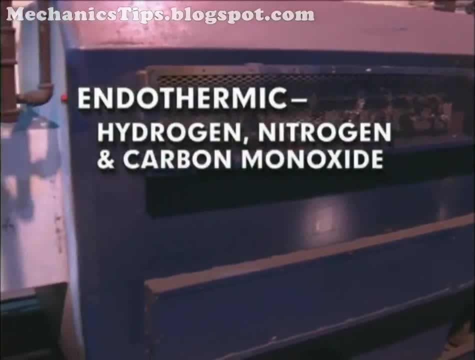 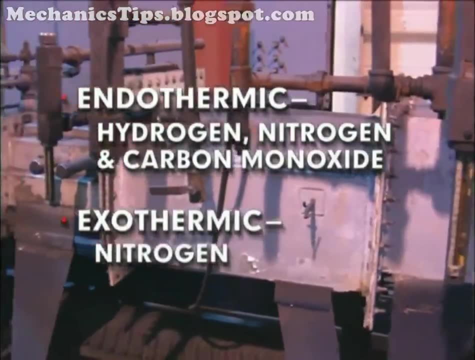 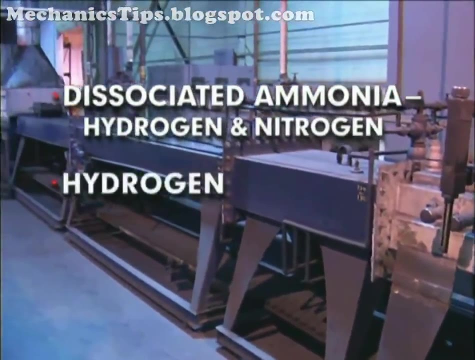 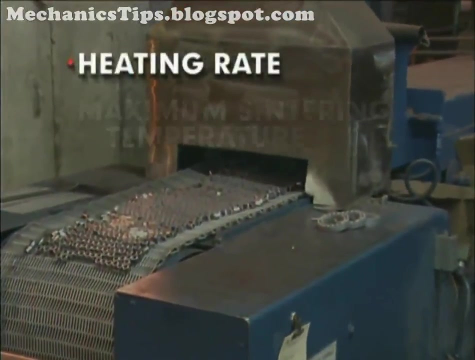 furnace may be: endothermic, which is composed mainly of hydrogen, nitrogen and carbon monoxide. exothermic, which is composed of nitrogen, mainly dissociated ammonia, which is hydrogen and nitrogen, or entirely hydrogen, vacuum or inert gas. to ensure proper sintering, the heating rate, maximum sintering. 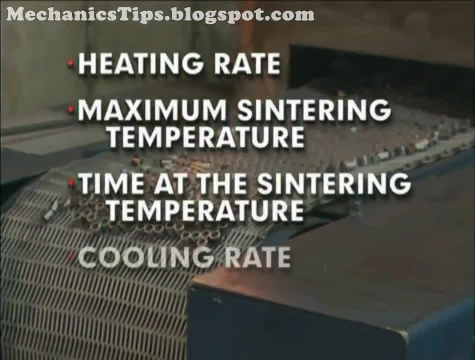 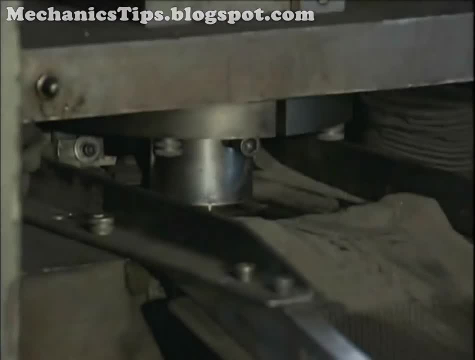 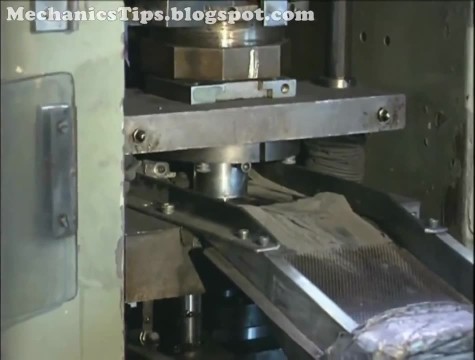 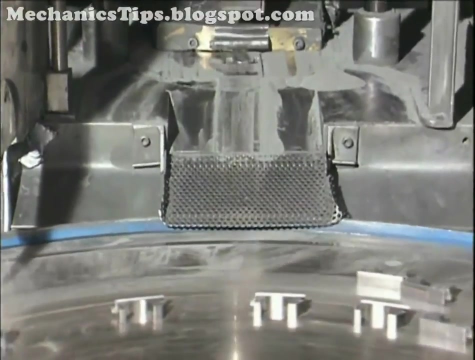 temperature, time at the sintering temperature, cooling rate and furnace atmosphere must be closely controlled. powder metallurgy is a metalworking technology used primarily for producing parts from metal powder. the primary advantage of powder metal parts is design flexibility. parts can be produced to net or near. 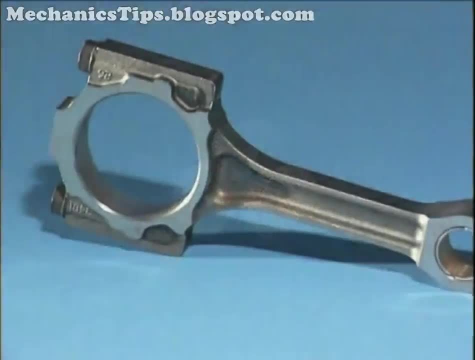 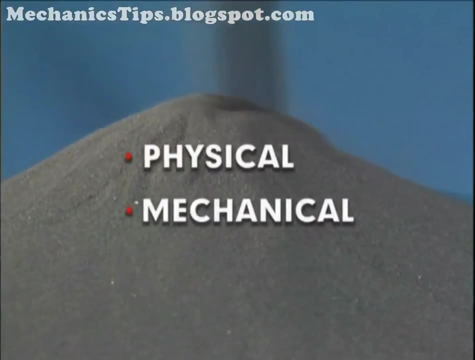 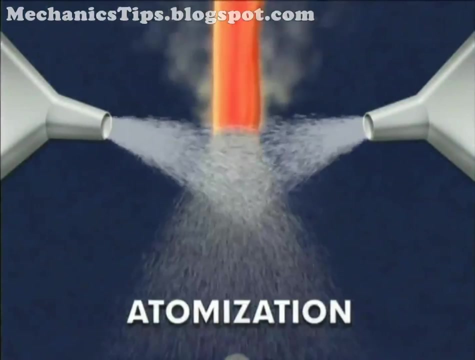 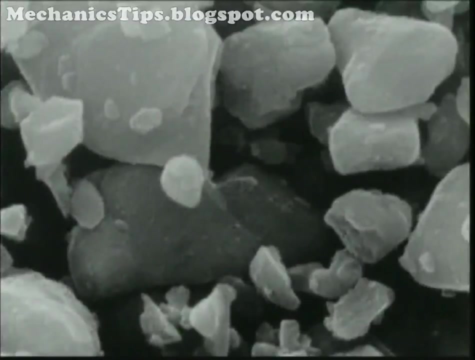 net shape and to controlled porosity or nearly full density. most metal powder is produced by physical or mechanical methods. atomization by high-pressure water or inert gas is the most common physical method. mechanical methods include milling in hammer and rod, ball grinding or attrition mills. metal powder used for parts production can be a combination of: 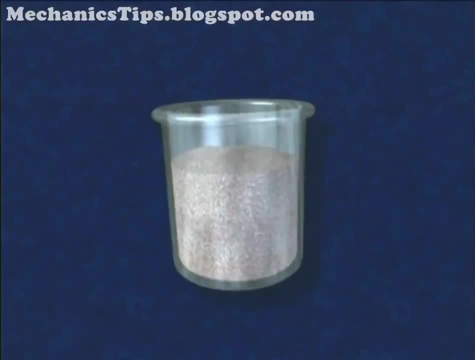 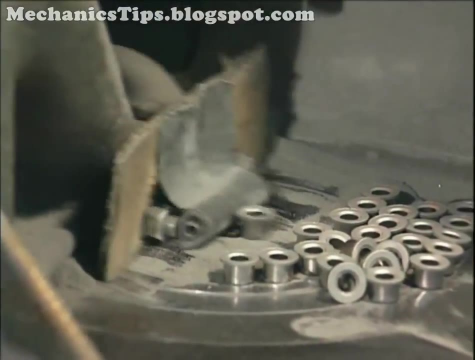 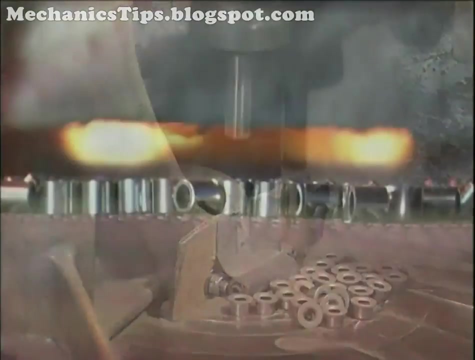 metal powder used for parts production can be a combination of various elemental particles or pre-alloyed powder. the powder is then consolidated in dyes or molds, shaping and densifying the powder into a compact of the desired park. the compact, which is in a green state, is then sintered. the common rule for using metal powder is that you must have a bowl of metal.